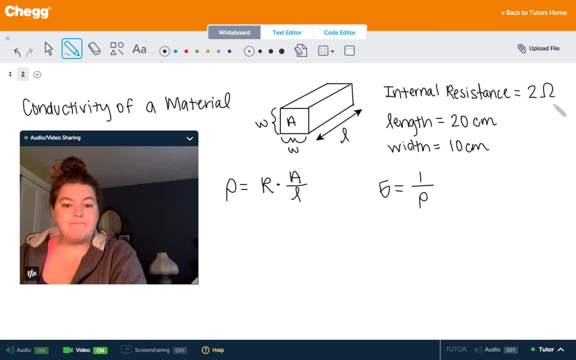 that has an internal resistance of 2 ohms, a length of 20 centimeters here and a width of 10 centimeters right here. Now you may recall, if you've ever had to calculate resistivity before or resistance from resistivity, that resistivity is equal to the internal resistance times. the 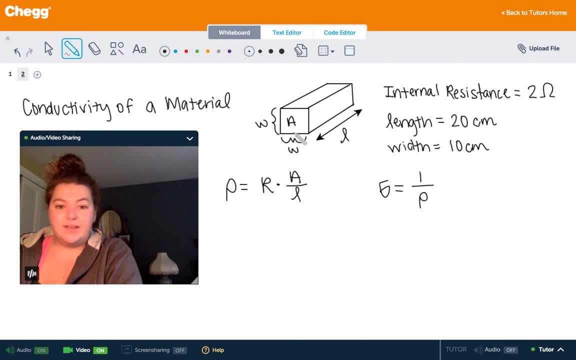 cross-sectional area, which is this square, right here in this material, divided by the length of material we're considering right here. So from resistivity we can find conductivity. So let's say we want to find the conductivity of this material right here. 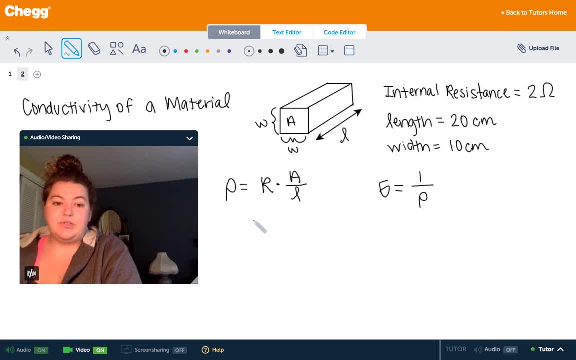 Well, we have the internal resistance, which is 2 ohms, and we have length and we have width of these sides of the square here. But we know that in SI units our resistance units should be ohms, and that's fine, That's what we have. But our distance units should be ohms, and that's. 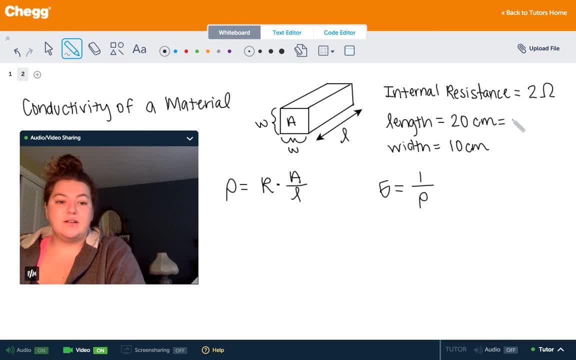 units should be in meters, So 20 centimeters is 2 tenths of a meter or 0.2 meters, And likewise, width, 10 centimeters is 1 tenth or 0.1 meters. Okay so, since we know that this is a square, the 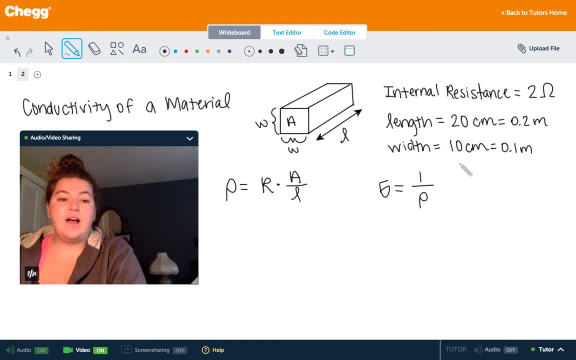 width and the width are the side lengths of a square. we can find the cross-sectional area as being um 0.1 times 0.1, or area of a square. 0.1 squared and 1 tenth squared is just 1 100th. So we: 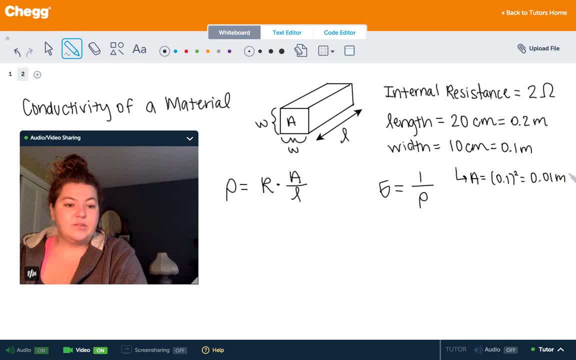 have 0.01 square meters. Okay, now we have everything that we need to find the resistivity of this material. So resistivity is equal to the internal resistance which we have to fill in the container. So we're going to have the resistance which is equal to the 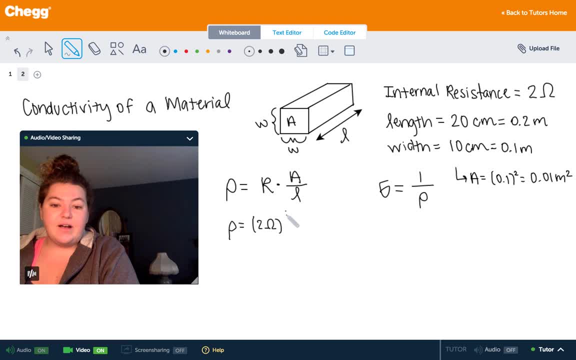 ohms times the area, we have 0.01 meters squared, and divided by the length, we have 0.2 meters, all right, so dimensionally we see that we have meters squared on top and meters on the bottom. so one of those meters is going to.